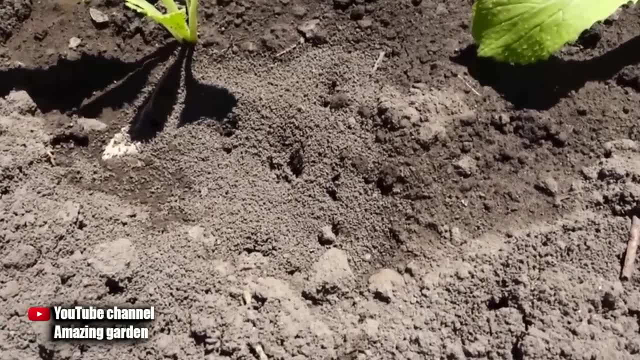 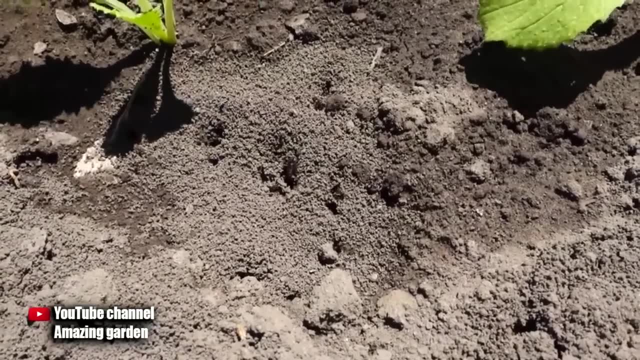 Hello friends, Today I will tell you about a simple folk remedy that will help rid your garden of ants. Now you see frames from last year's video in which I used sugar and boric acid. I will leave a link to it in the upper right corner in the tips. At the moment, a year later, 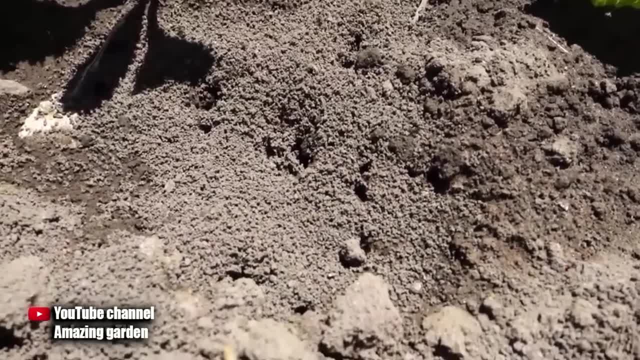 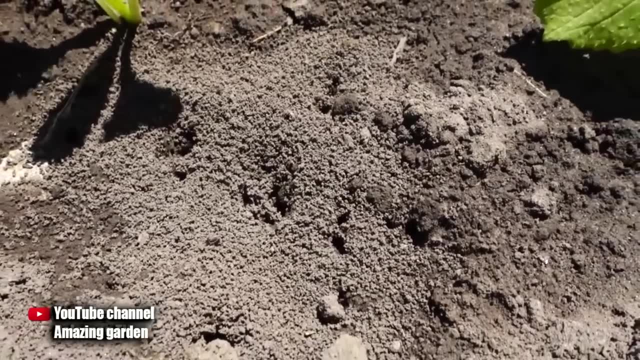 there are no ants in my garden. This tool worked quickly and 100%, But in the comments under this video there were people who wrote that this remedy somehow did not attract their ants. Consequently, the ants did not eat the bait and these people could not bring them out. 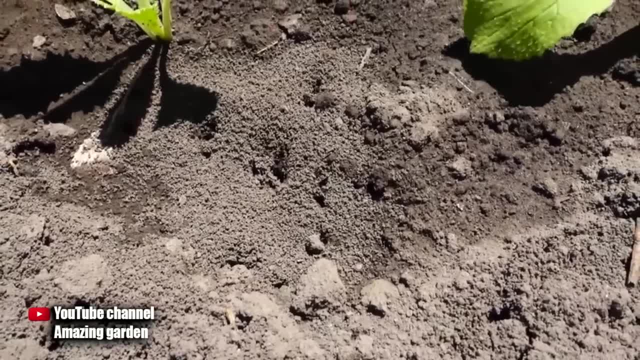 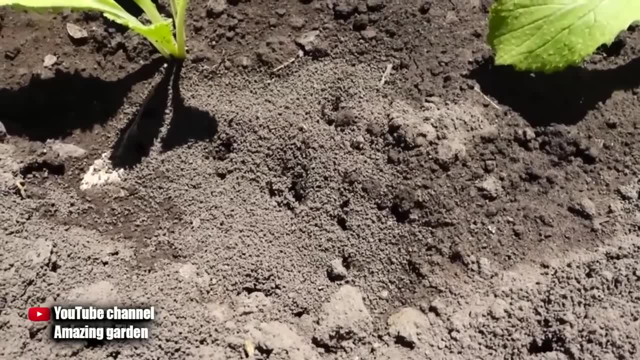 And now I will tell you about such a bait that the ants will defy, nightly smell, eat, take it to their anthill and feed everyone with it. There will be no trace of the investigator from the anthill. The recipes are quite simple: You will need two boiled eggs. 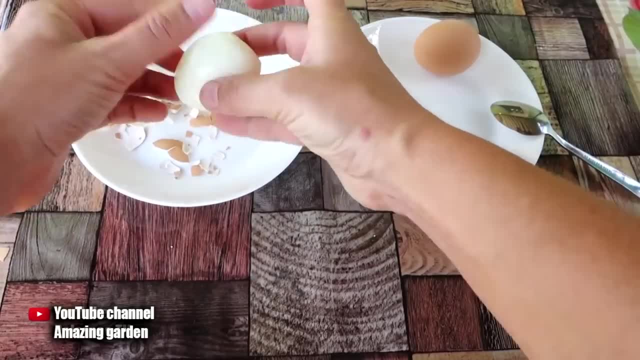 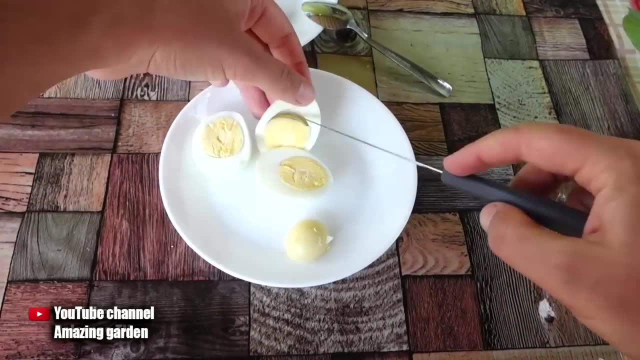 they need to be shelled and the proteins separated from the yolks. We don't need proteins. they can be used for food and the yolks are just right for this bait. As the smell of yolks, ants will come out of the bait. the ants will be able to eat the bait. The ants will be able to eat the. 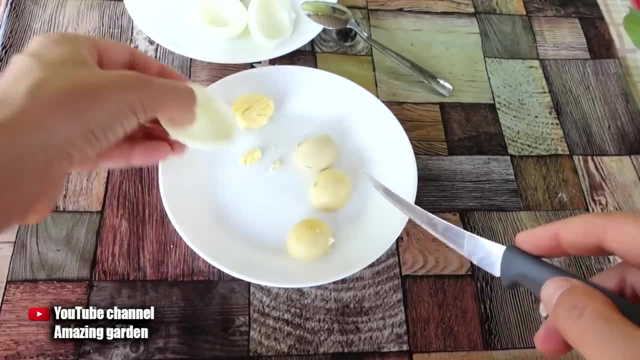 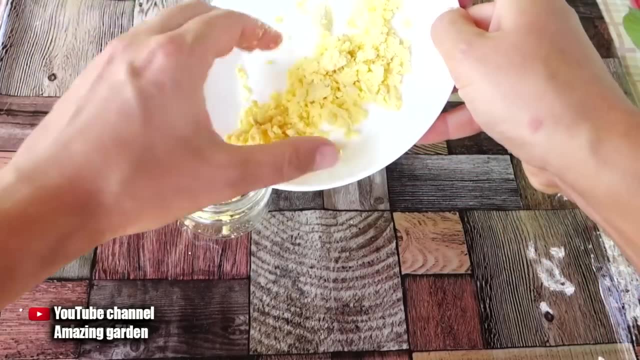 bait and come running very quickly. This has been proven over the years. Then mash the yolks with a regular fork. to mash them, Then you need a small container. You can take a glass jar with a twist In which we will prepare the bait And since we will not use everything at once, 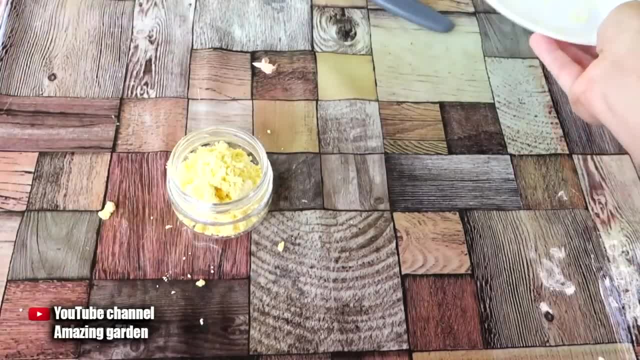 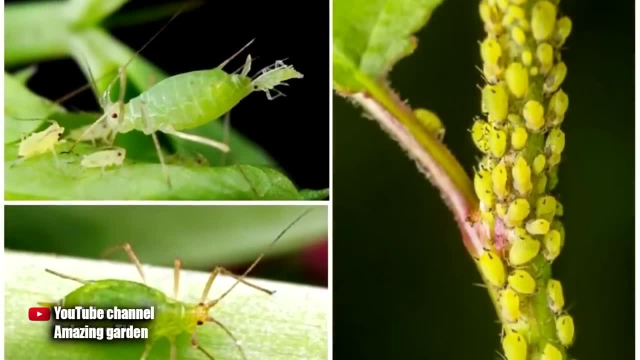 the bait can be stored for some time. Pour the yolks into a jar. In addition to the fact that ants love egg yolk, we will strengthen the bait with honey Because ants have a strong sweet tooth. they are garden pests, Because aphids live in our garden. They suck the juice from young leaves, thereby destroying the young growth and the plants themselves, And the discharge from this aphid is sweet. Therefore, the ants run on them. And since the ants understand that aphids give them such sweetness, they spread it to all. the trees and plants in the garden, thereby increasing their numbers. Accordingly. ants themselves are not pests, but are accomplices of aphids that destroy our garden. One has only to destroy the ants, then the aphids will immediately disappear. This has already been verified. I add a teaspoon of honey, Then I add the main ingredient. 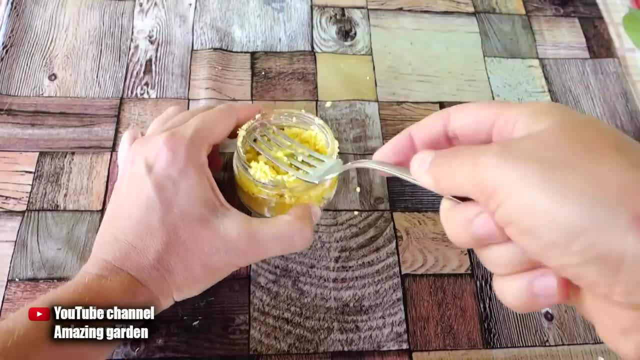 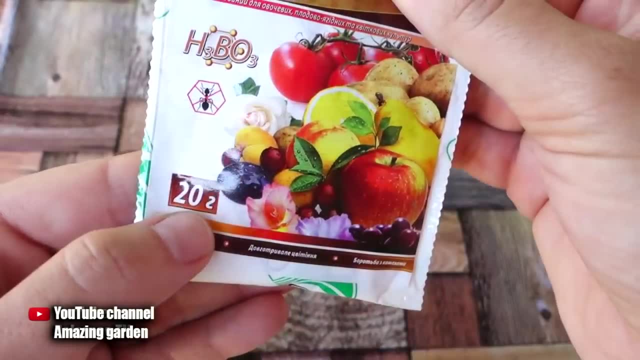 it is boric acid. It is sold in pharmacies, but one like mine is sold in garden stores. It can be used not only in the fight against ants, but also to feed garden plants. I think you will immediately have a question: is it possible to use liquid boric acid? my answer is: